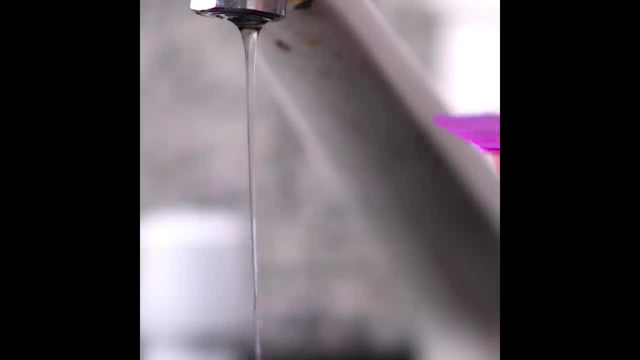 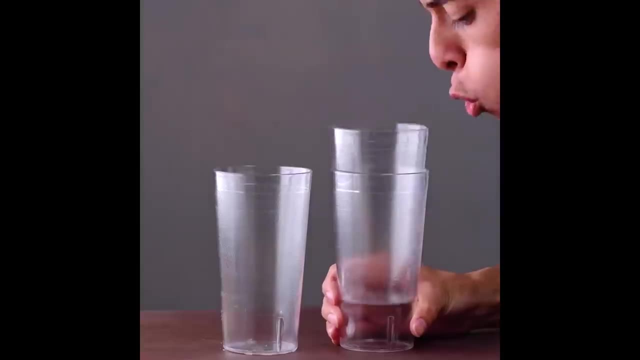 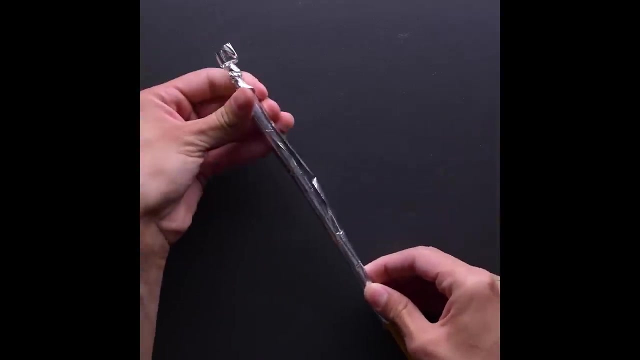 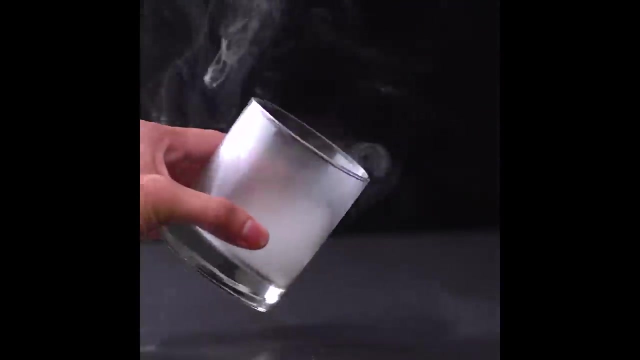 Hello everyone, welcome to my channel. Today, I will show you how to make a simple and easy-to-understand bookmark. First, I will show you how to make a bookmark. First, I will show you how to make a bookmark When you create a bookmark. 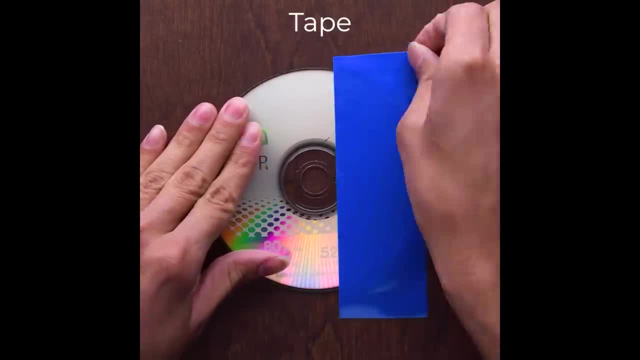 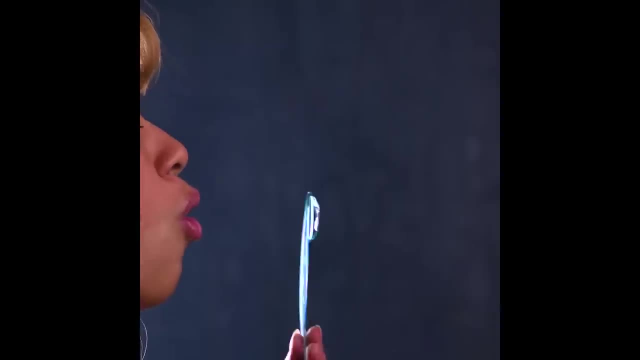 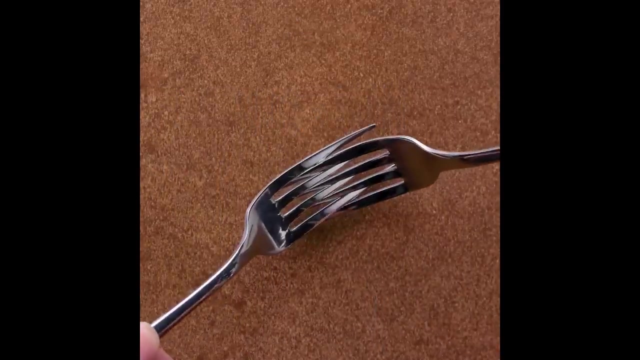 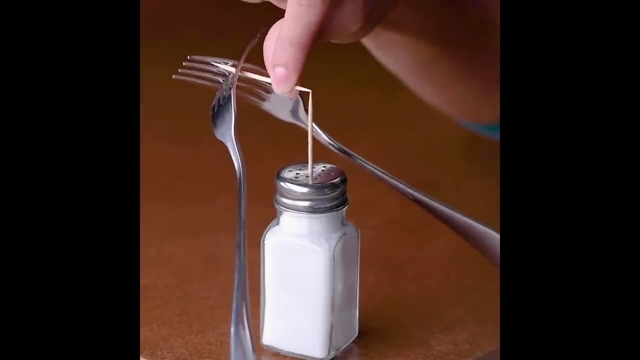 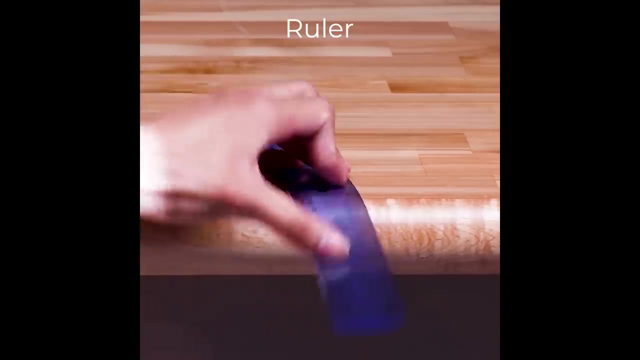 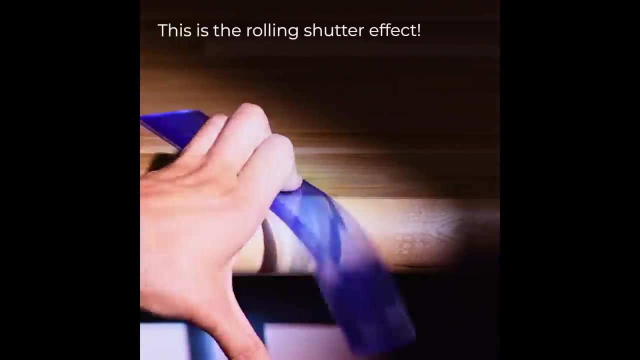 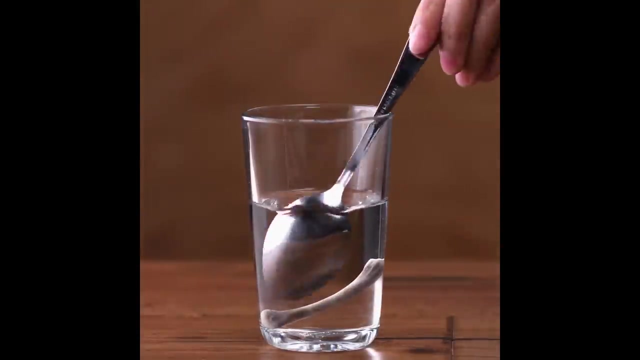 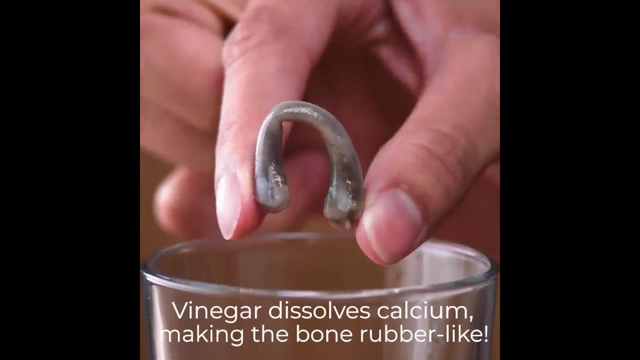 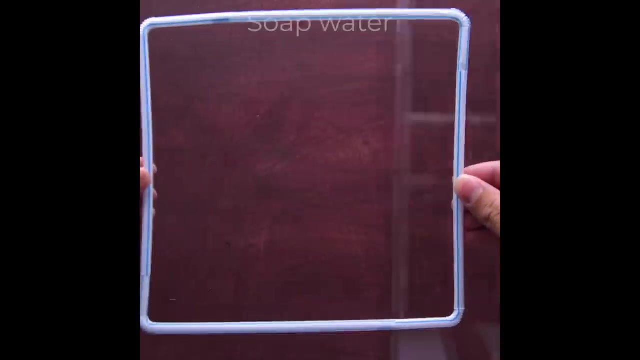 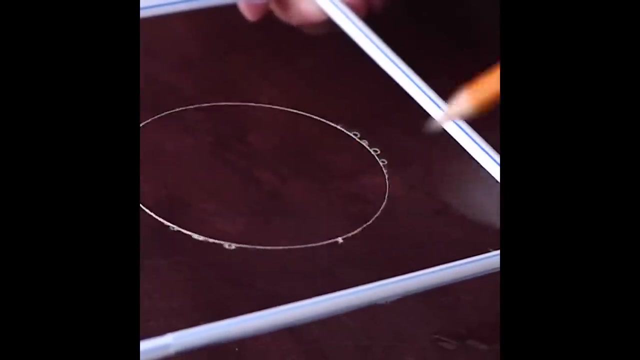 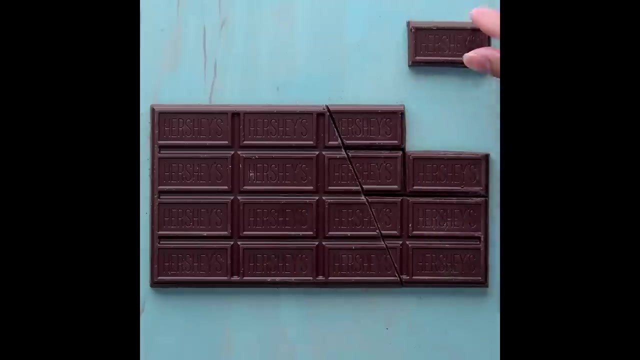 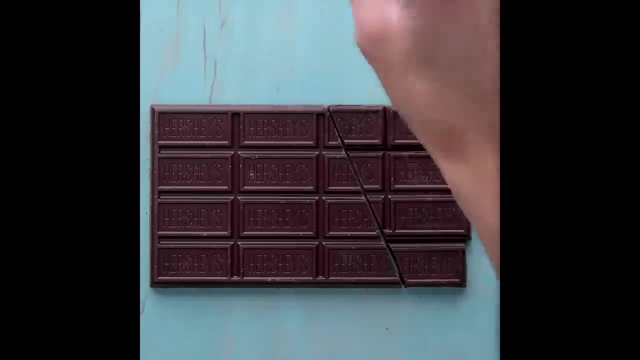 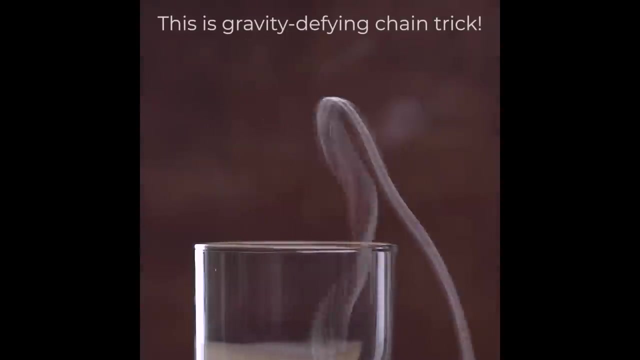 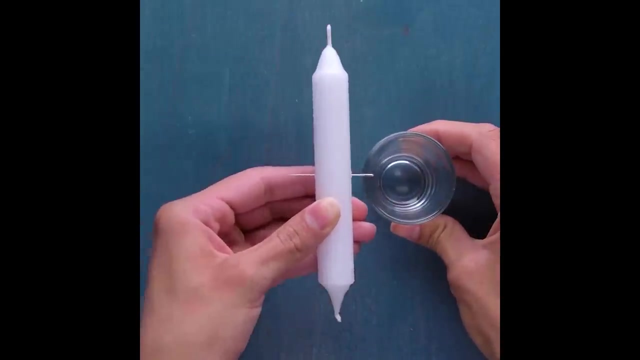 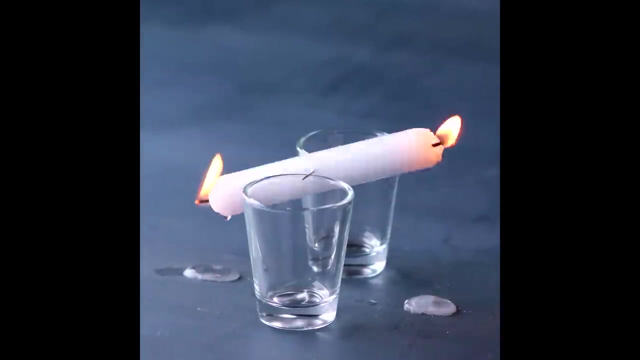 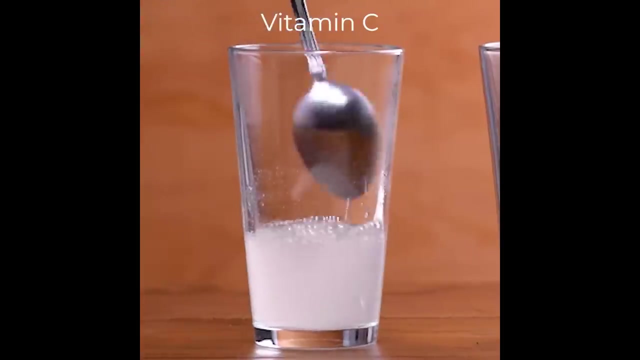 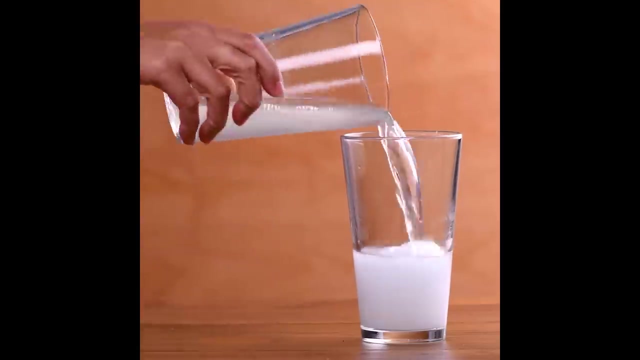 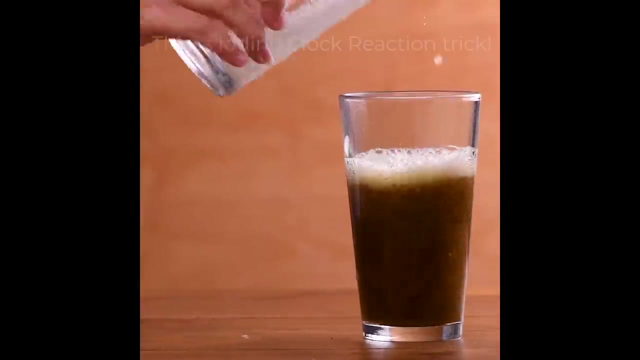 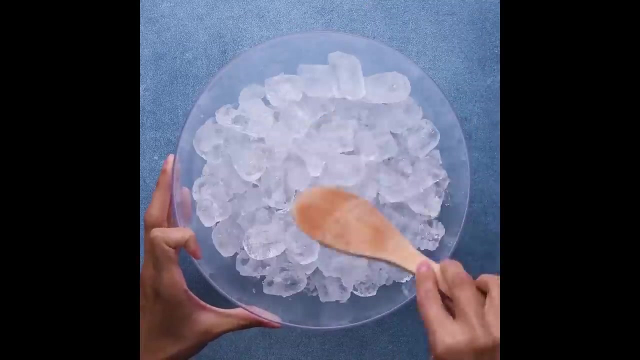 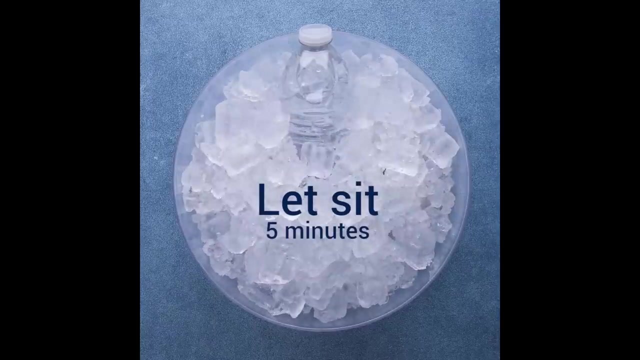 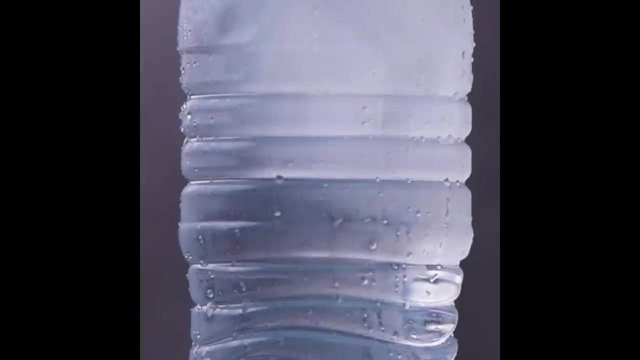 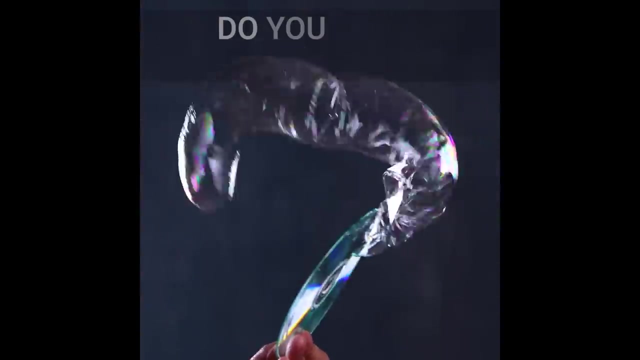 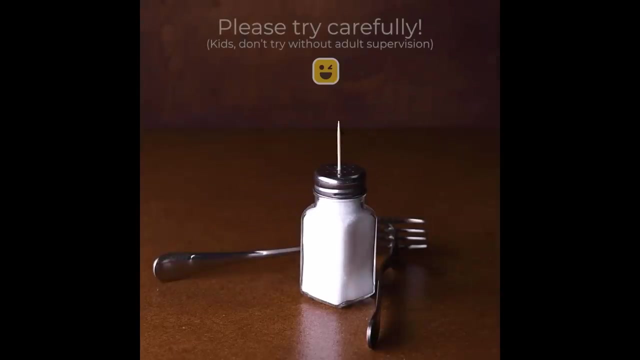 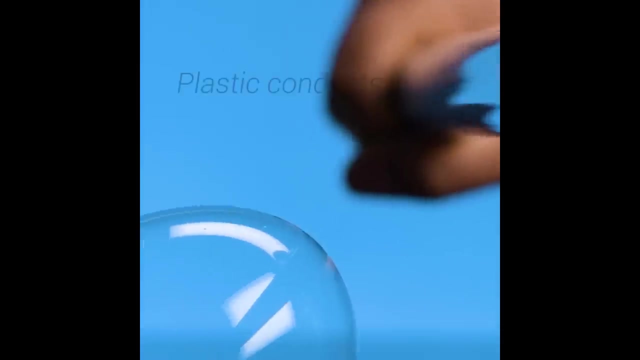 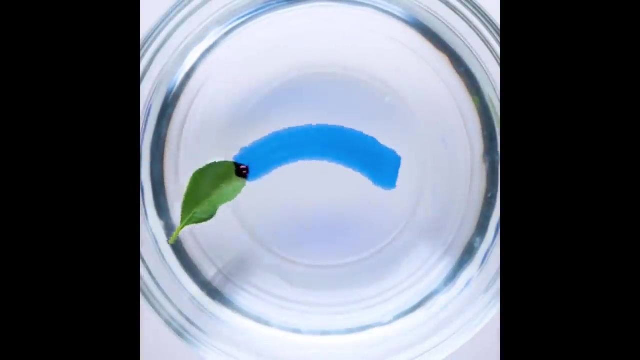 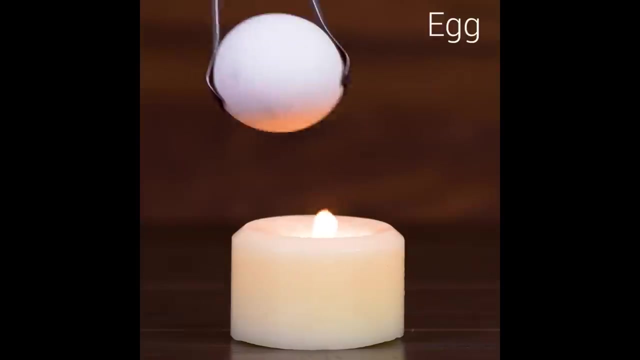 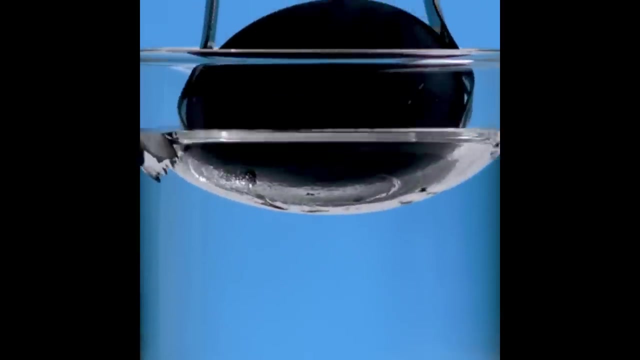 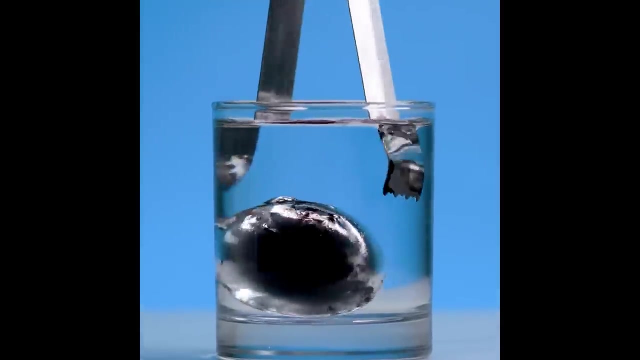 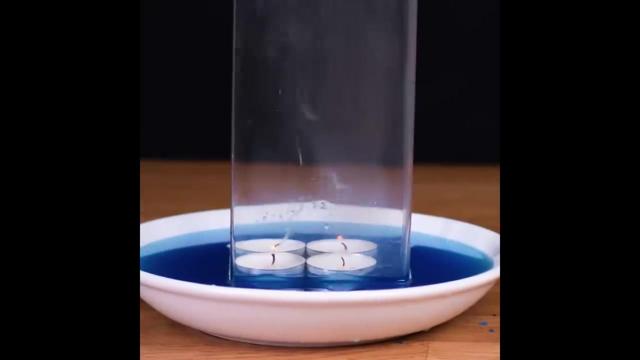